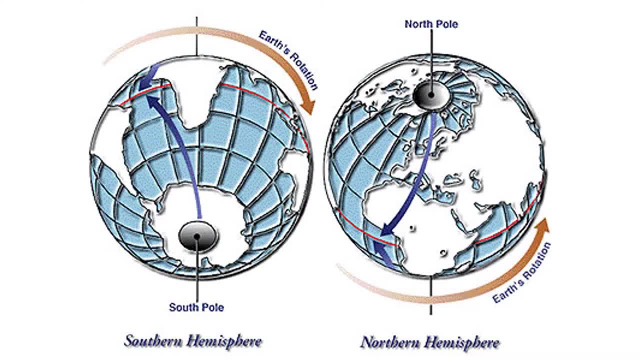 more complicated. The Earth's spin creates a deflection of these air movements. The counterclockwise spin of the Earth causes a deflection to the right in the northern hemisphere and to the left in the southern hemisphere. This is known as the Coriolis effect. The Coriolis effect. 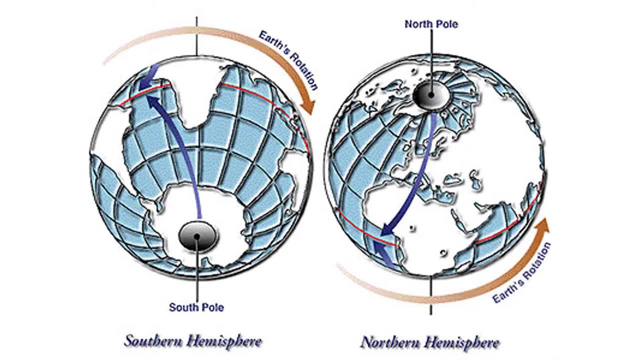 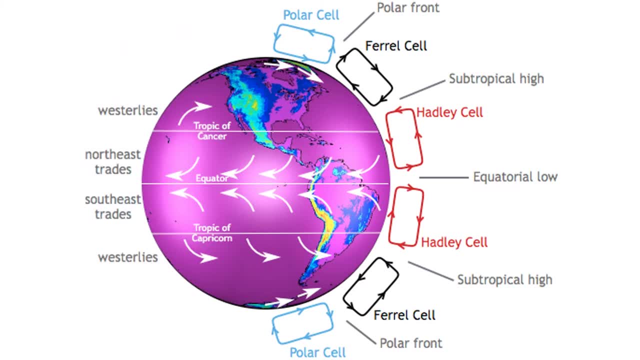 has a much stronger influence at higher latitudes than at the equator due to the difference in speed of the rotation at the different latitudes. The differences in air pressure and the Coriolis effect combined create three atmospheric cells north and south of the equator. These 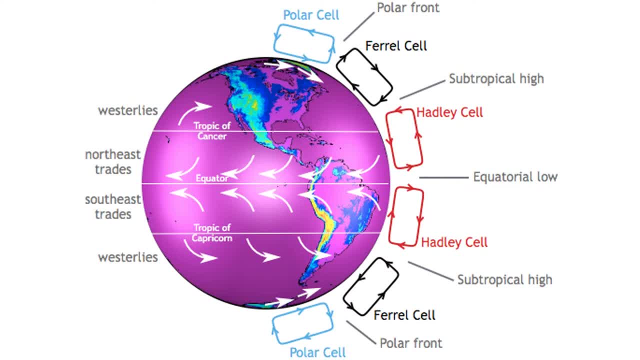 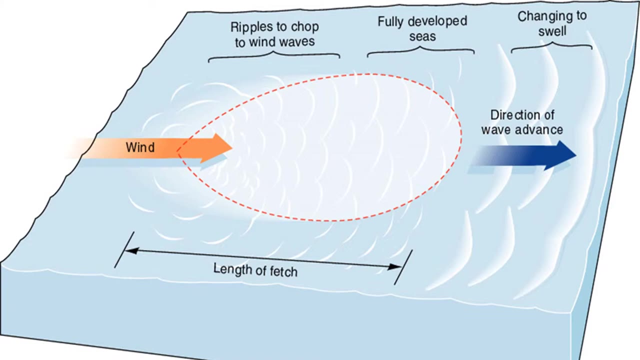 are known as Hadley cells, Ferrel cells and Polar cells. These atmospheric cells create our northeast and southeast trade winds and our westerly wind systems. The wind is the mechanism which translates the energy from the sun to the surface of the oceans. Put simply, as the winds blow across the ocean surface, the wind will blow. 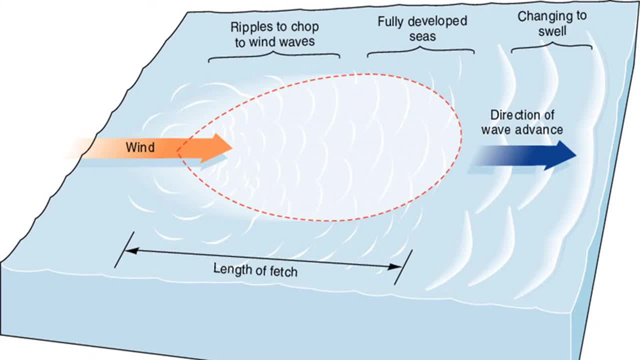 up. The friction generated produces small surface waves, increasing the surface area caught by the wind and so increasing the friction and size of the wave. Of course, it is not quite as simple as this in reality. When we consider the Coriolis effect, we will see. 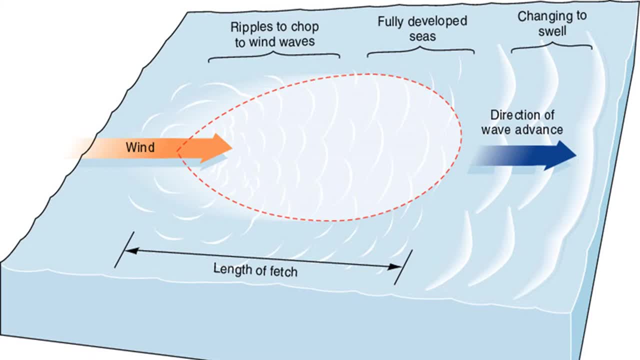 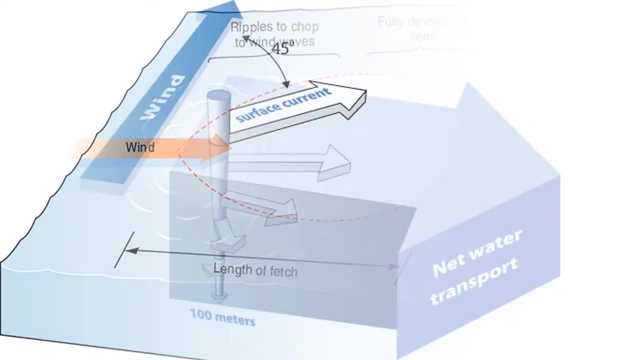 that over a period of time, the surface current will be deflected, just as the air was to the right in the northern hemisphere and to the left in the southern hemisphere. As the wind pushes the surface water in one direction, the wind will push the surface. 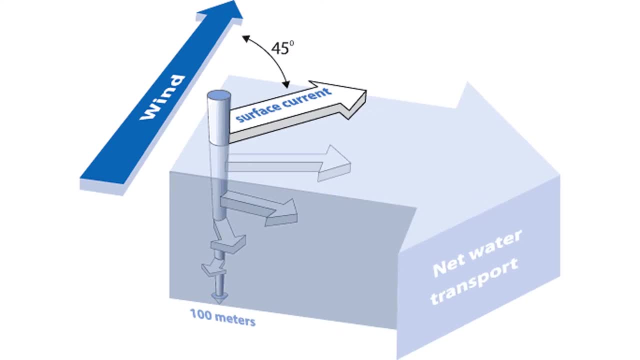 water in the opposite direction. The wind will push the surface water in one direction. the Coriolis force pushes the surface water to the right. The result of these two forces acting together is a movement of surface water at 45 degrees to the right of the wind direction. 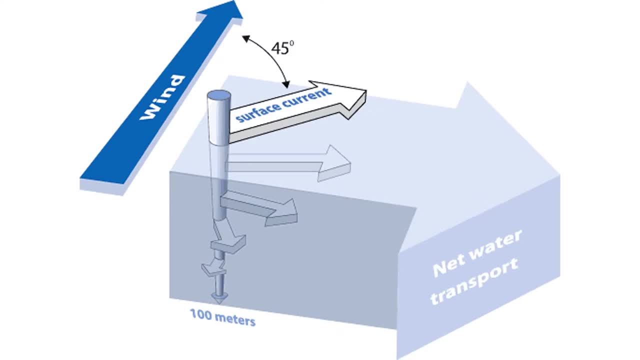 The movement of the surface layer acts on the layer below it, and so does the Coriolis effect. In each layer, some energy is lost and the angle of deflection slightly increases. This continues down through multiple layers of water, creating a downward spiral known. 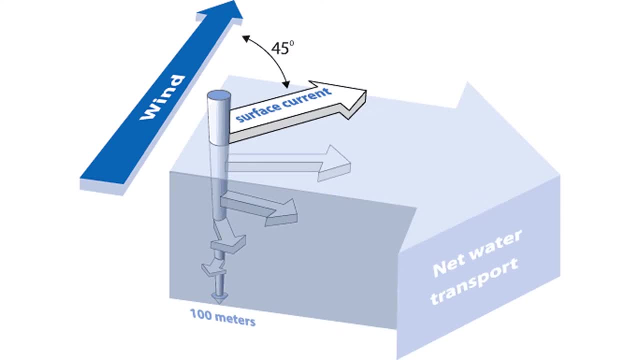 as the Ekman spiral. Once the spiral reaches a certain depth, the effects of wind and Coriolis act in direct opposition at 180 degrees of each other, and an Ekman current is created, flowing at 90 degrees to the right of the wind direction, depicted by the broad arrow in this slide. 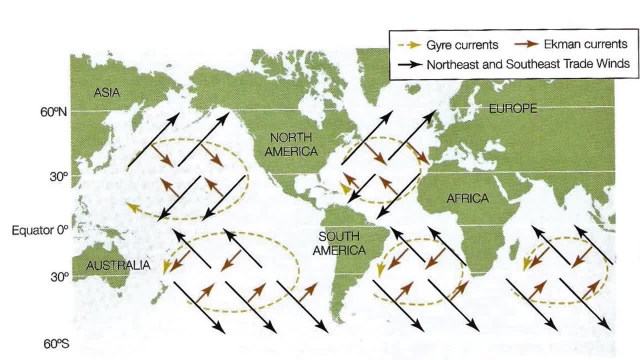 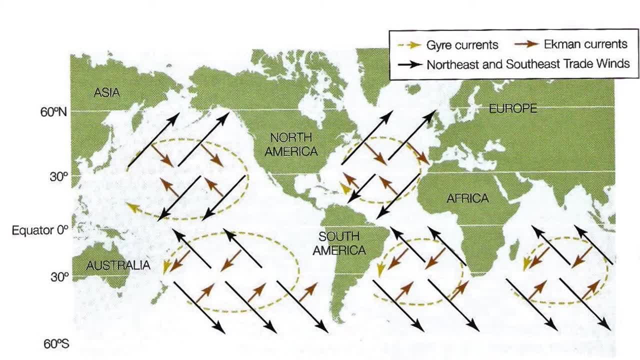 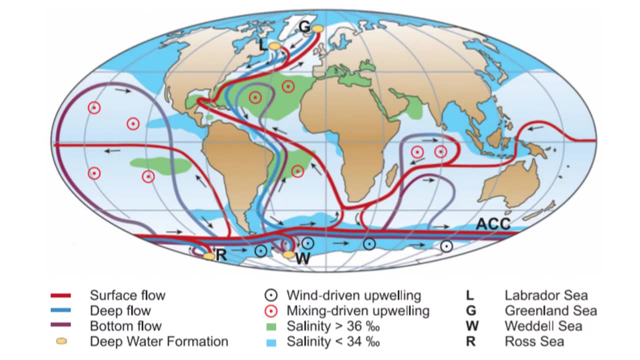 successful spiral. Eventually, the water in the centre is forced downward below the Ekman layer, where they spread laterally and are again affected by Coriolis force, causing a clockwise gyre, generally known as a geostrophic current. As well as the surface currents, there is a second mechanism driving the large scale. 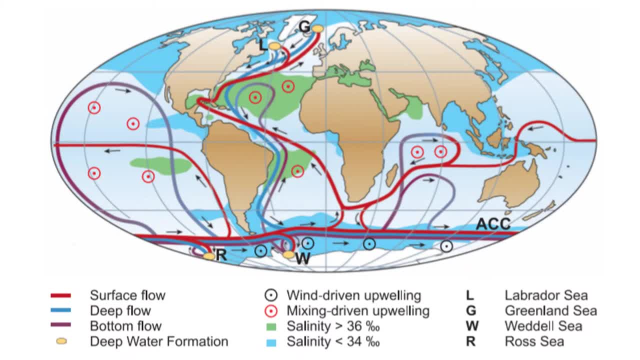 movements of the oceans. This is called thermohaline circulation. Thermohaline comes from two Greek: Thermal haline. circulation is part of the large-scale ocean circulation driven by global density gradients caused by surface temperature and freshwater fluxes. It begins at the poles, where surface waters are cooled, increasing. 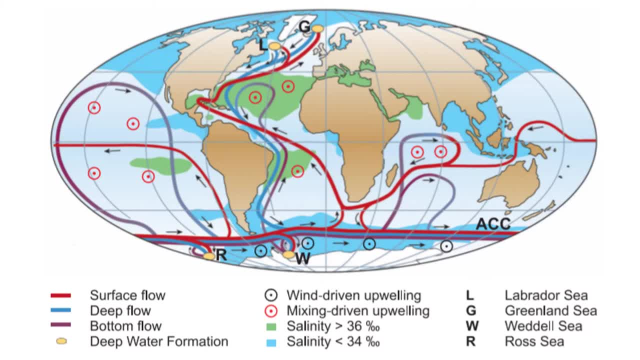 their density. Once cooled enough, these surface waters sink, forming deep and bottom waters. The deep and bottom water slowly spreads towards the equator. North Atlantic deep water, combined with bottom and deep waters from the Antarctic, spread throughout the oceans, eventually upwelling to the surface again, where 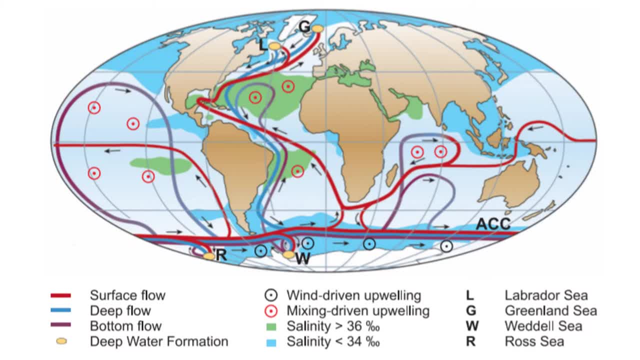 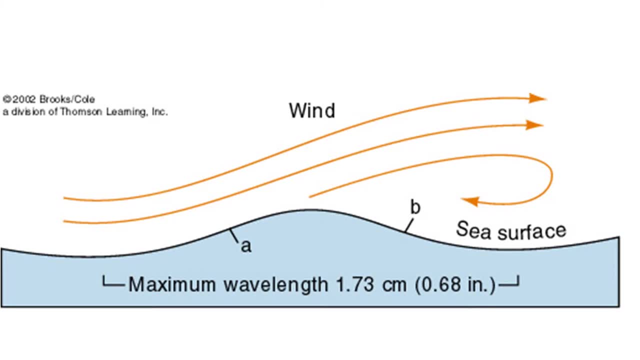 they are driven by surface currents back to their formation sites. This whole circulation process is known as the Great Ocean Conveyor Belt, As was briefly touched on earlier in this film. small waves are created by wind acting on the surface waters. Here we will take a look at waves in more. 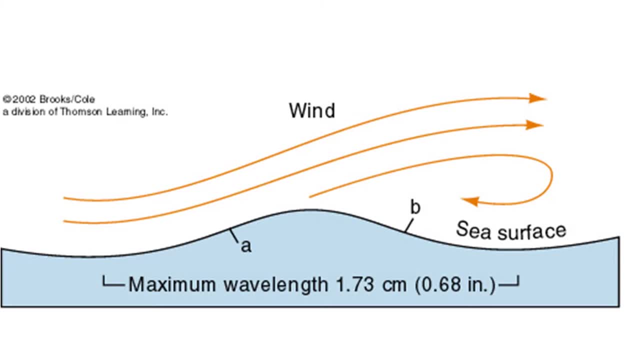 detail. Waves are the result of a disturbing force and a restoring force acting in opposition. Small surface waves created by wind energy are called capillary waves. Capillary waves are classified as having a wavelength of less than 1.73 centimetres. At this point, the restoring force is the surface tension of water. 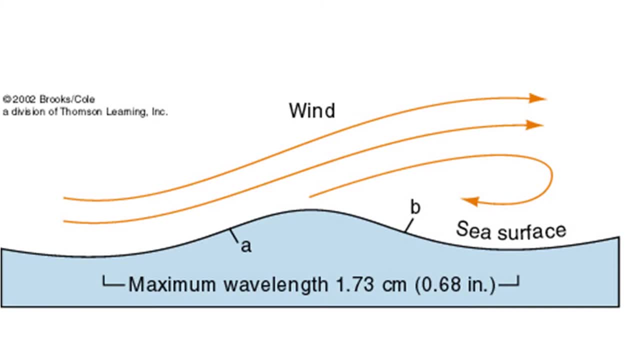 Once a capillary wave grows beyond 1.73 centimetres, the surface tension is broken, The restoring force changes to gravity and the wave becomes a surface gravity wave. As the crest of a surface gravity wave falls, its momentum causes it to land in a new position. As the wind acts on these waves, they continue to. 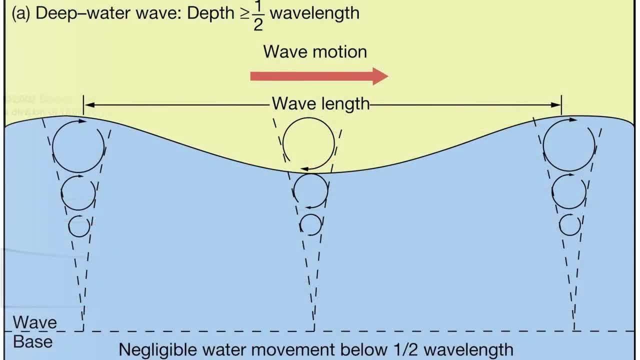 move away from their point of origin. Contrary to what you may picture, it is the flow of energy moving through the water. we observe, not the actual movement of water. The water itself actually moves in a near-perfect circle known as a wave orbit. These orbits are not just confined. 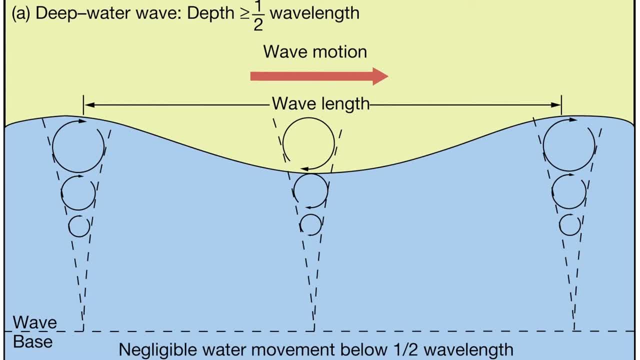 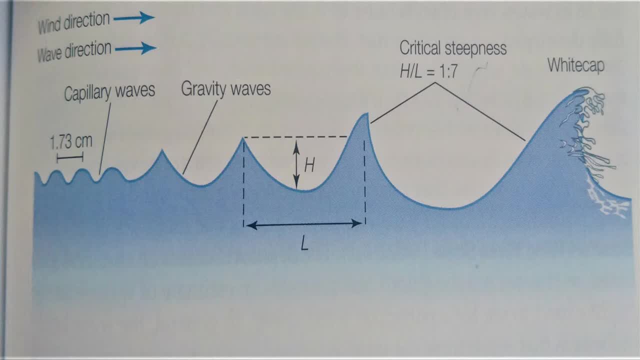 to the surface layer, but propagate down through the water column, getting smaller with depth. There are shallow, intermediate and deep-water gravity waves, and they are classified based upon the depth of water relative to the size of the wavelength. A deep-water gravity wave is one where the water depth is greater than half of the wavelength. 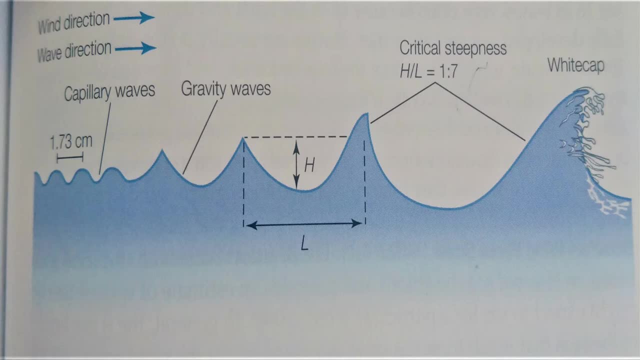 In this instance the bottom does not interfere with the wave orbits. As the wave approaches shallow water, it becomes an intermediate gravity wave. Here the orbits are disturbed and the speed of the wave is affected. When the depth is less than 1- 20th the wavelength, the wave becomes a shallow gravity wave. The height of a 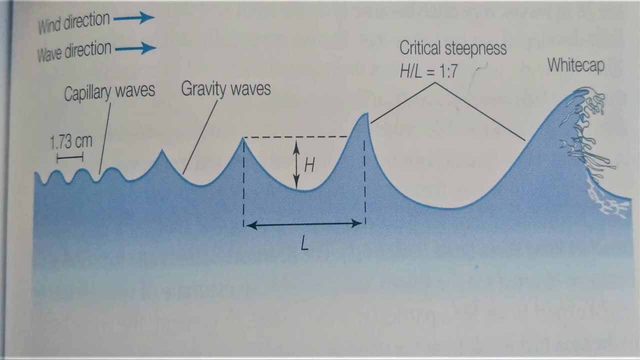 gravity wave builds more quickly than its wavelength. As a result, a surface gravity wave will eventually collapse or break. This critical steepness occurs when the height reaches seven times the wavelength and the breaking wave is known as a white cap. At this point, the energy input from wind and energy 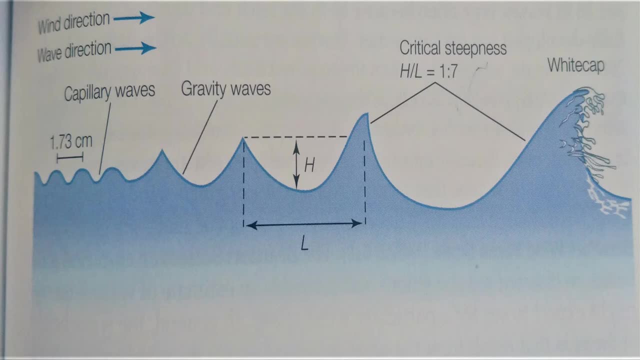 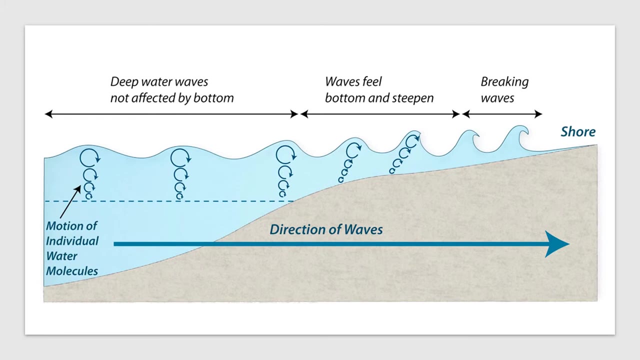 dissipated from the white caps, is at equilibrium. As deep-water gravity waves are approached the coastline, the water depth decreases, causing it to transition to an intermediate and then shallow water gravity wave. As the wave is slowed, the waves following behind catch up building height Once the depth is around 1.3 times the height of the 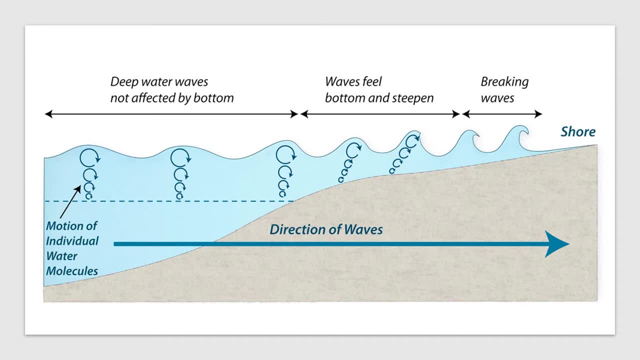 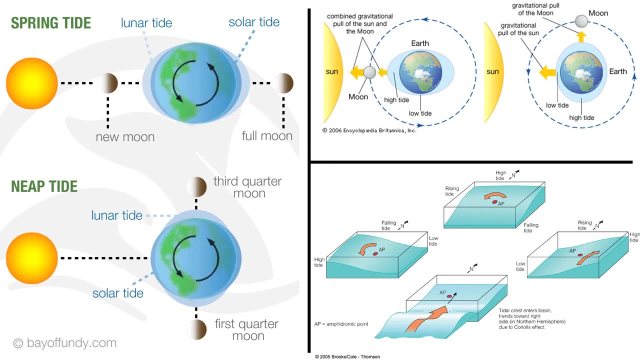 wave it will break. These breaking waves are known as surf. The tides can be described as the largest waves on the planet, as they ebb and flow in the same way a small wave does. They are the result of gravitational force caused by the Moon and Sun. As the Earth, Moon and Sun move, 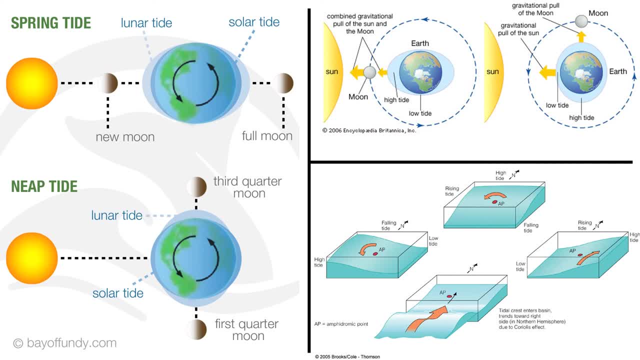 around relative to each other. altering gravitational forces pull on the oceans, causing our tidal variations or, as we more commonly know them, high, low spring and neap tides. Around the globe, there are lunar or semi-dianal tides occurring twice in a day, and solar or dianal tides occurring once in a day. As the names,